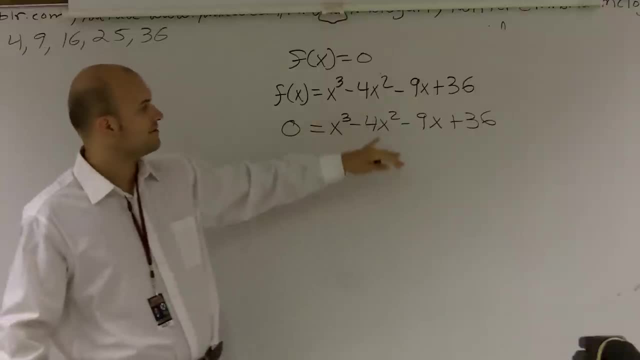 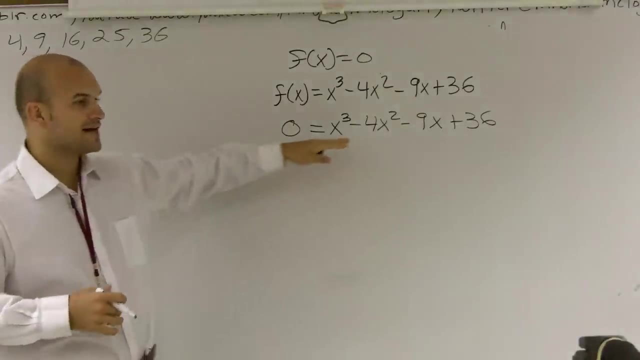 Here we have a lot of stuff going on. We have x cubed, a negative 4x squared and a negative 9x. So we have a lot of x's And we can't use our regular factoring, because that was always. when we're dealing with a trinomial, when it has three terms or a quadratic, We were always so used to doing your factoring and setting it up as far as two linear factors. So now we need a different kind of factoring method. Well, the factoring method we're going to want to use and always you should look at this: whenever you see four terms, you should always look into factoring. 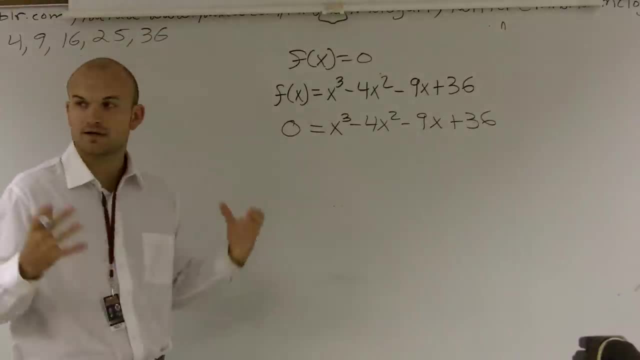 By grouping. So what you really just want to do is just kind of take two different terms and see if you can bring them together and if we can factor something similar out of them. So in this problem, I'm just going to look at these first two terms and I'll say: all right, is there something that these two have in common? You can say, yes, I can take out an x squared out of here. So if I factor out an x squared, I'll be left with x minus 4.. And then here are these two terms: If I took out a negative 9,, I'd factor out a negative 9.. 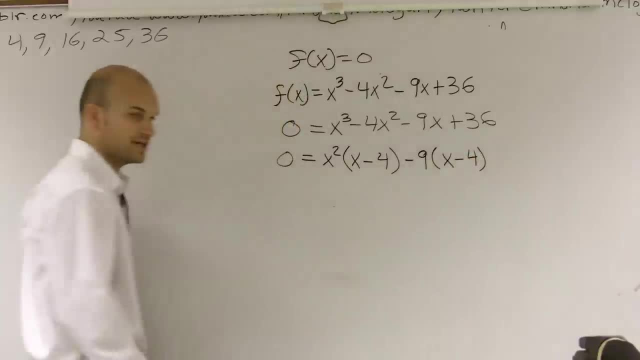 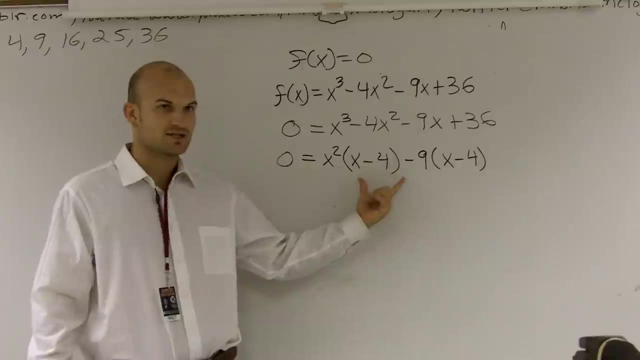 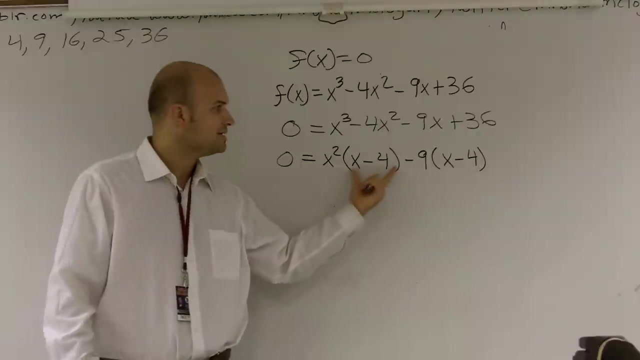 I'll be left with x minus 4.. Which again gives me to what I want when I'm looking to factor my grouping. Because now, if you look at these, treat these just as another term. I know they're a binomial, They have two terms within them, but just treat these just like a regular variable. You can now both of these terms, this and this, both share an x minus 4.. So what I'm going to do is I'm going to factor both of those out. So if I factor out an x minus 4, I pull it out. 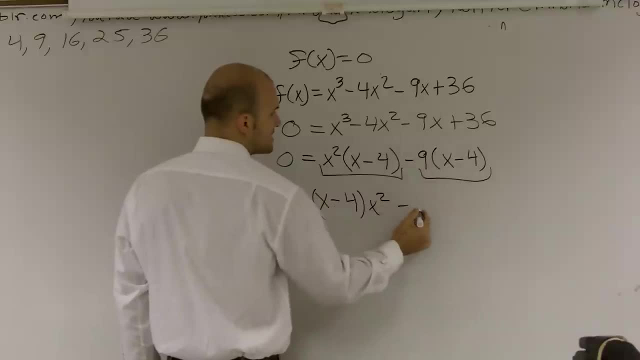 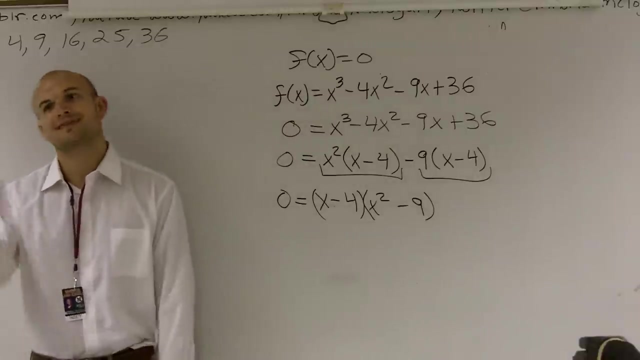 I am left with an x squared, And if here I factor out an x minus 4, I'm left with, sorry, a negative 9.. Does everybody understand that? You raised your hand, Good, Thank you. Why is it that we have two x minus 4s? Why did we almost drop it? 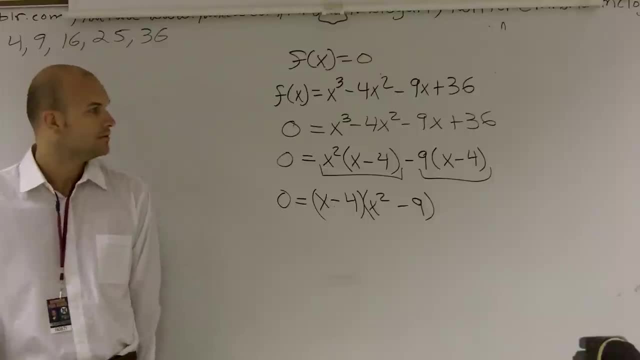 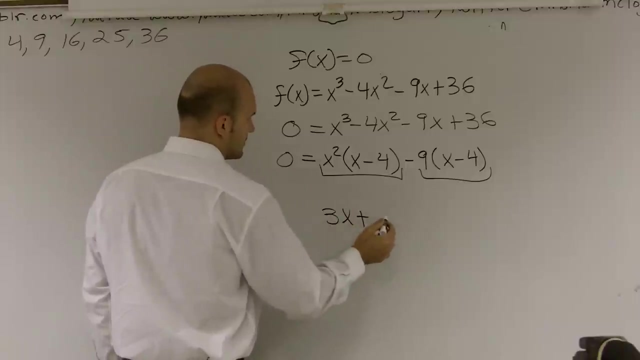 What do you mean? why did we almost drop it? Because we have two x minus 4s, Two x minus 4s and then an x minus 4 is only one of them. Ys are only one of them. Okay, what I'm doing is it's like this, It's like 3x plus very square right. What can you kind of factor out of this? 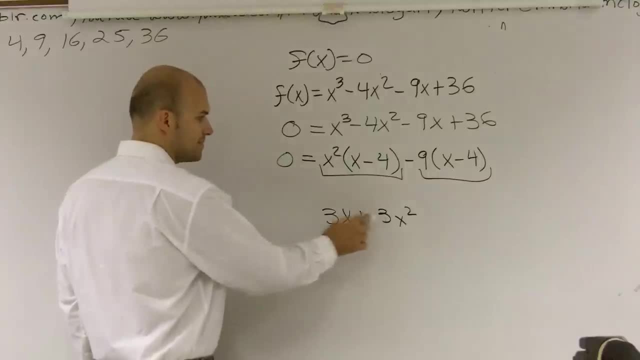 3x. You can factor out a 3x, right? So what I'm doing is I'm pretty much you're kind of saying you have like these three actually Yeah. So what I'm doing is I'm taking a 3 out of both of them, right? 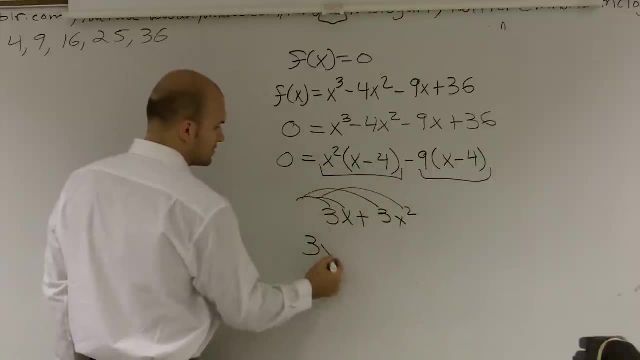 Yeah, And I'm taking an x out of both of them. So you're left with. so what's left? Well, that's a 1 plus x, correct? Well, that's the exact same thing I'm doing here. These both share an x minus 4.. 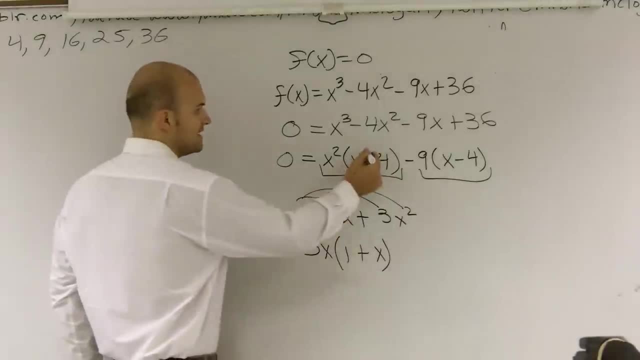 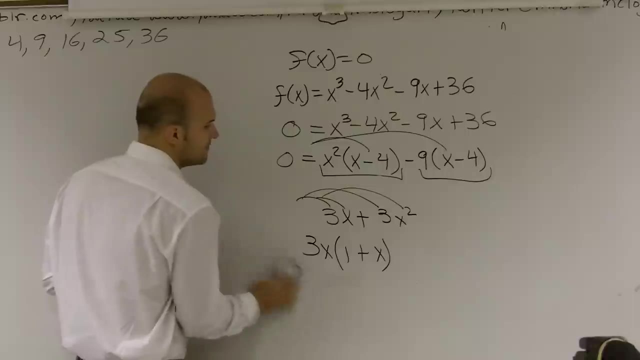 Just treat it like it's another variable. So I'm taking an x minus 4 out of both of them. So therefore, that's why I only have when I take an x minus 4 out of both of them, I'm just left with an x minus 4.. 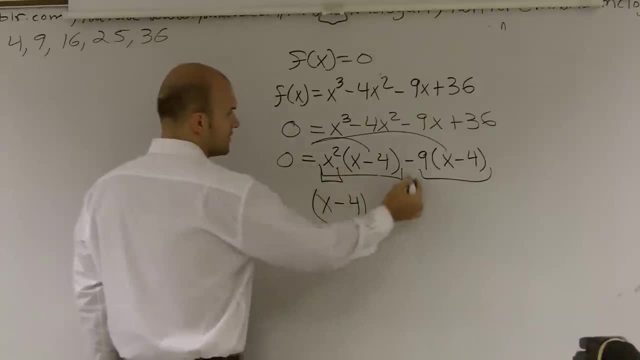 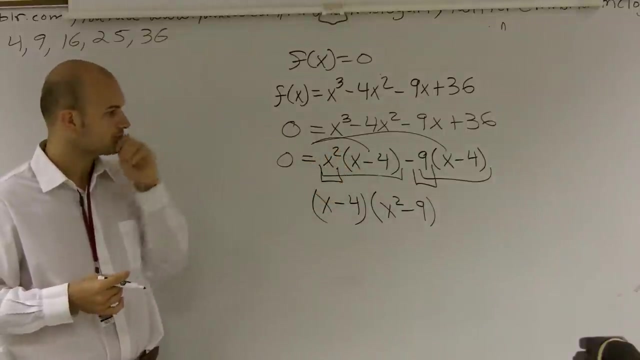 So then, what's left over? Well, that's left over and that's left over. So that's why I write that in its own parentheses: x squared minus 9.. Does that make any more sense? Yeah, but I was just curious, because when we did the work, 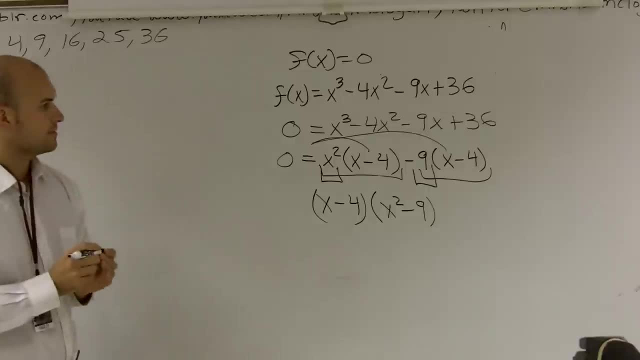 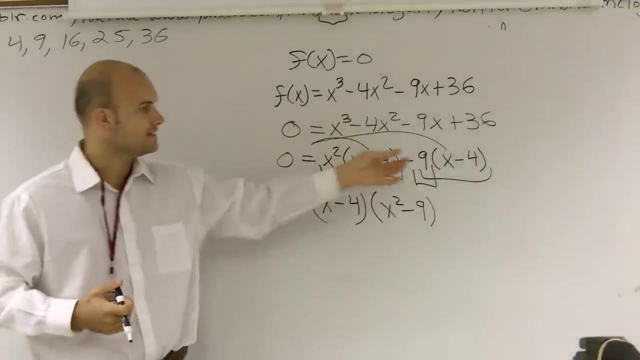 it was almost kind of like we were dropping one of the ones in parentheses. So I was just confused: Yeah, you're not dropping it. What you're doing is you're actually factoring it out. You're actually you're taking these two x minus 4s and you're actually you're factoring out. 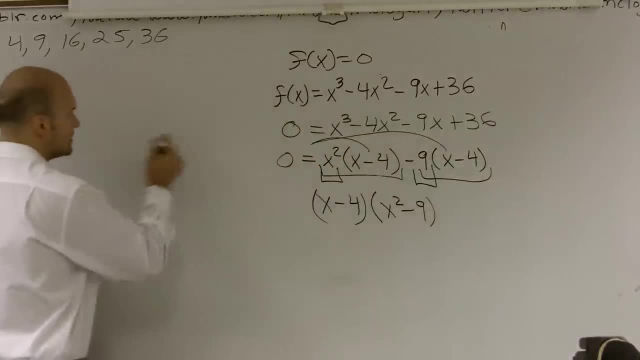 you're pulling it out and then whatever's left for it. I mean, it's the same thing if yeah, well, I'm trying to think of a different example of your 3s, but if you just remember that you know, if you look at these, what do these two share?